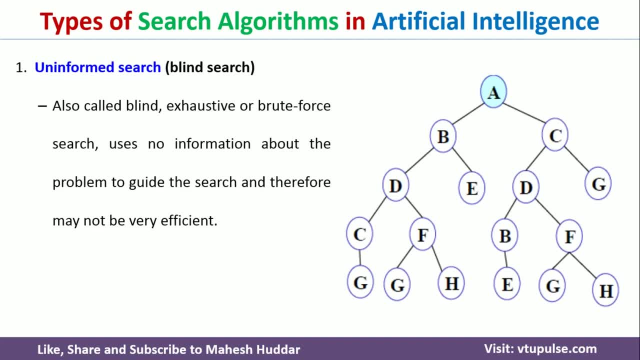 informed search, also called as heuristic search algorithm. First we will try to understand uninformed search algorithm. In uninformed search algorithm, given a state, if you have multiple number of paths, it will not select a path which is having a least cost. or you can say that the 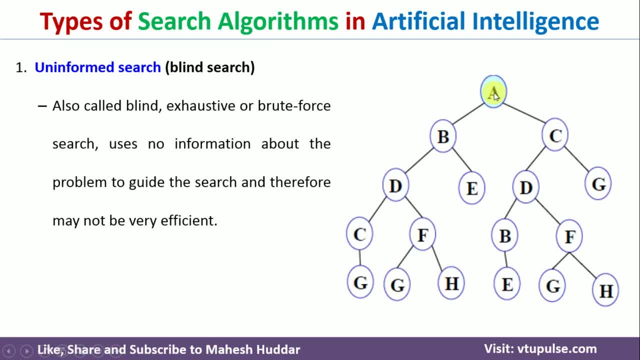 optimal path. It will go to each and every path and then it will try to get the goal state over here, For example, in this case- let us say that right now we are present in this state A- There are two paths are there? Either we can go to this particular B and then we can go to this particular 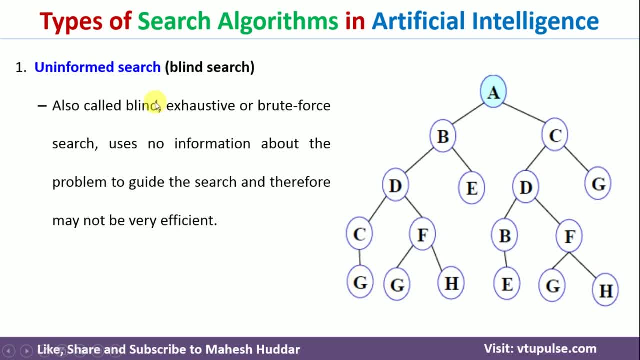 C to reach this particular goal, state G here. So in uninformed search technique it doesn't apply any logic or something like that. It will choose one of this particular thing and then it will try to go to this particular goal state over here. So if it goes through this particular path, 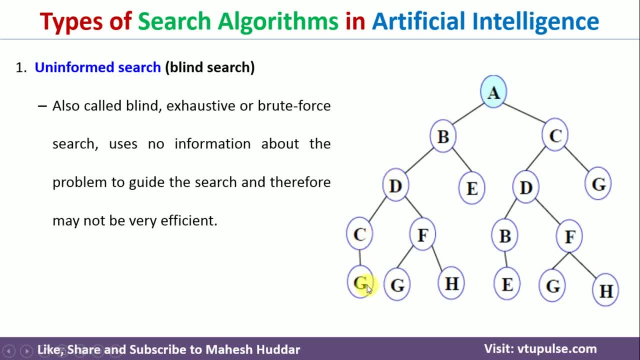 let us say that A to B, B to D, D to C and C to G, it will go to the lengthiest path over here, But if it has gone to this particular side, that is, A to C and C to G, it would be the least cost path in this particular case. 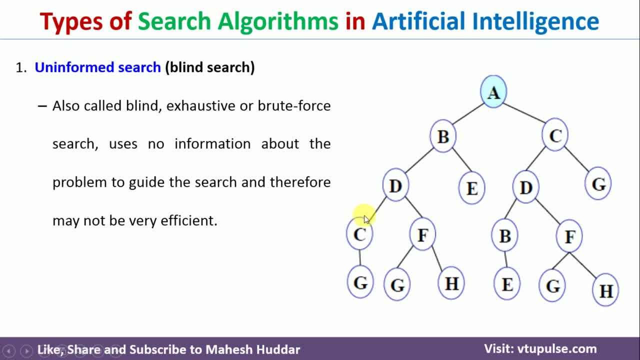 But it will not apply any logic here and then and it will just follow up one of this particular path and then it will try to reach this particular goal state over here. So that is the reason it is called as uninformed search technique. Now coming back to the second one, and that is called as: 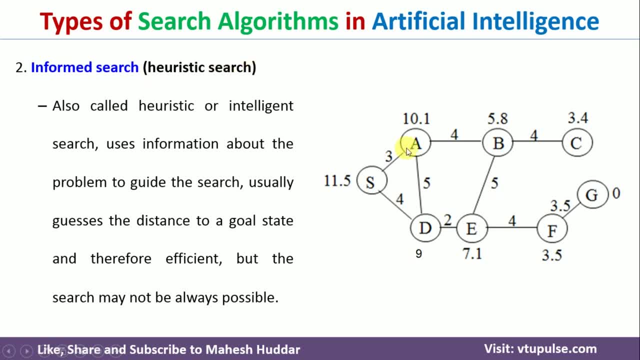 informed search, or it's also called as heuristic search. So whenever you are present in a particular state and there are multiple paths are there from that particular state, it will use some heuristic function and then, based on that particular thing, it will make a decision. Should I choose the first? 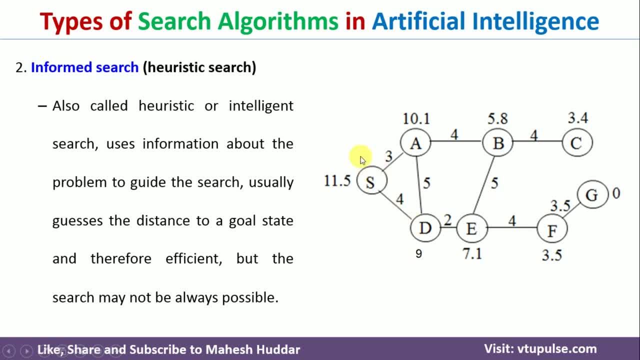 path, or should I choose the second path? So that is what the main thing happens in this informed search technique. So just to understand, let us assume that right now we are present in this particular state. Yes, there are two paths, are there? Either we can choose this particular. 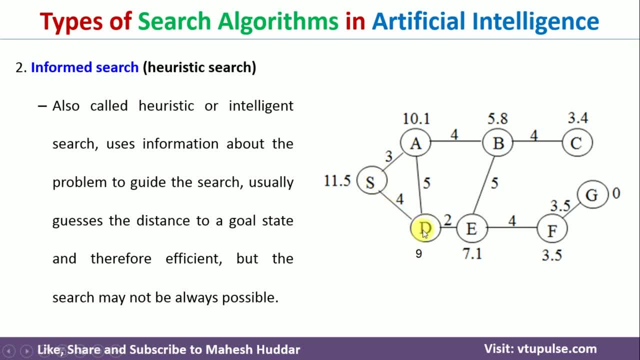 path to go to this particular A or towards this particular path we can select so that we can reach this particular D. For this one, we have the cost 3 and for this one we have cost 4.. Now there are multiple informed search algorithms. are there Just to explain this particular informed search? 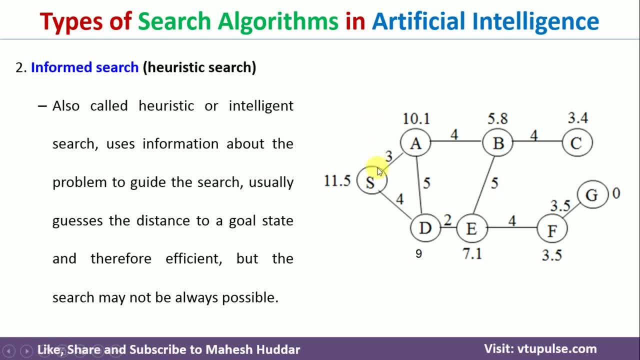 technique I will consider A star algorithm. So what A star algorithm does is it will take this particular cost plus it will consider the heuristic value. This one is called as a heuristic value, that is, 10.1.. What is this 10.1 is? it is a probable distance to reach from A to goal state. here. 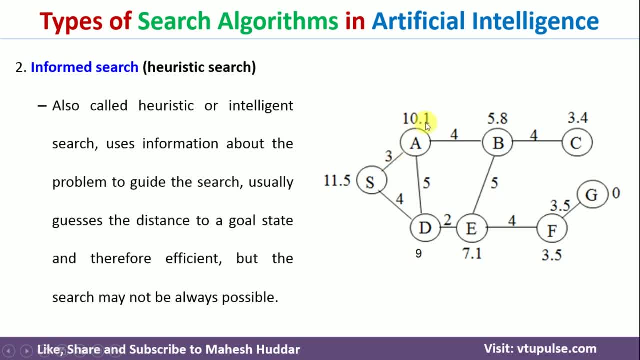 So this particular D plus 10.1, it will become 13.1.. So that is the heuristic value of this particular path. Similarly, we need to calculate this heuristic value of this particular path, that is, 4 plus 9, it will become 13 in this case. So if I choose this particular path, it will be. 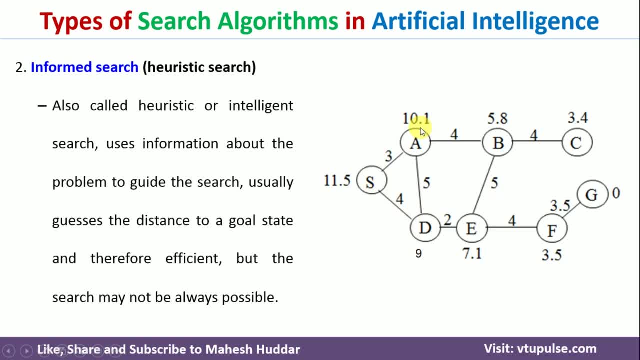 13.. If I choose this one, it will become 13.1.. So at this particular point of time, this will be the better option. over here Now it will go to this particular D again. it will try to find a suitable path so that it can reach this particular goal. state. 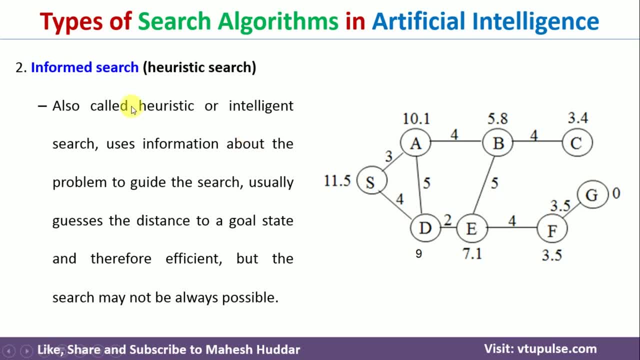 With a minimal cost over here. So this is how the informed search algorithm works. I have discussed this particular algorithm in detail in another video. we just go through that particular video to understand the completely how A star search algorithm works. Now these particular algorithms, that is, informed and uninformed search algorithms, were again categorized. 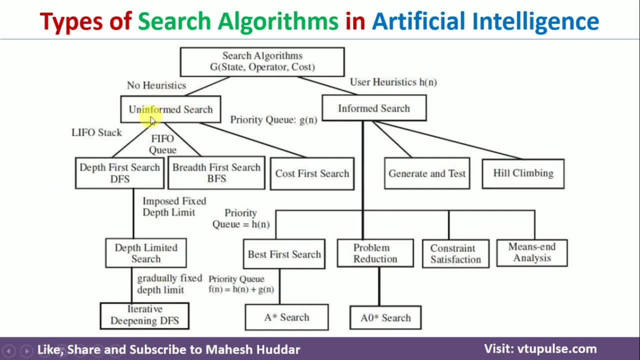 into multiple number of algorithms And informed search techniques were divided into three groups. one is called as depth first search algorithm If the implementation is done with the help of LIFO, that is, stack. Second one is a breadth first search algorithm, if the implementation 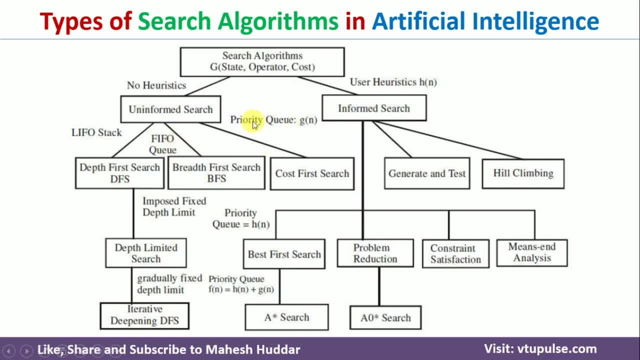 is done with the help of Q or FIFO. If priority Q is used, such kind of algorithm is called as a cost first search algorithm. in this case, Again, this depth first search algorithm is divided into two things, based on the depth limit. Whenever you set the depth, for example, 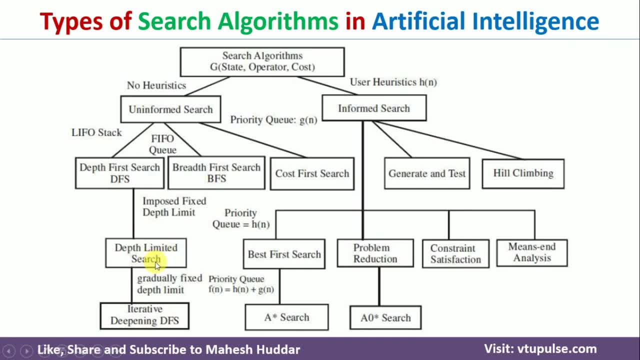 is equal to two or something like that, it will become a depth limit search over here. Again. if you go on increasing that particular depth from two to three, three to four or something like that, it will become iterative deepening depth. first search algorithm over here. 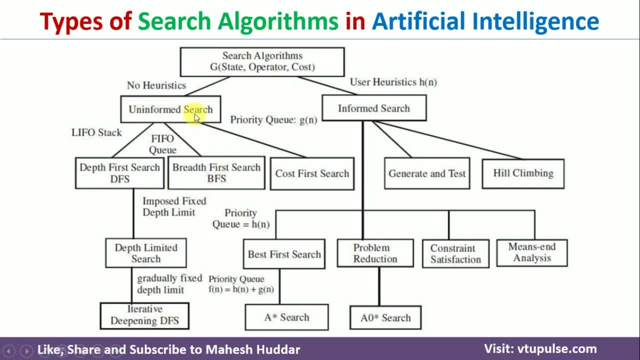 So these are some of the different algorithms which comes under this particular uninformed search. Coming back to informed search algorithm, they were categorized into mainly three groups. First one is generate and test. Second one is hill climbing. Third one is again into different groups. over here, Best first search algorithm: problem reduction algorithm.